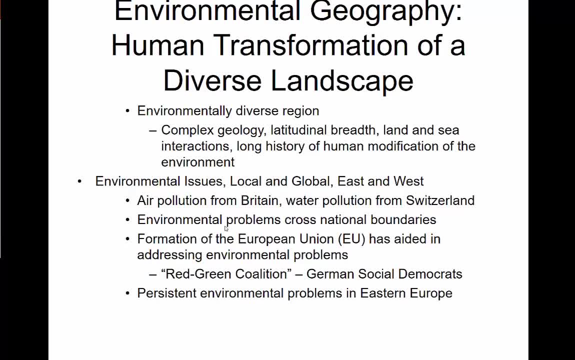 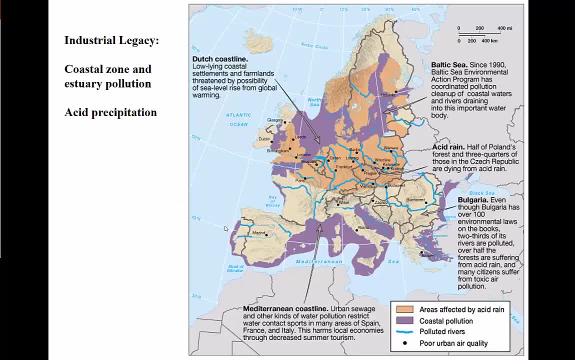 Environmentally diverse. It's got a complex geology, Issues with air pollution, water pollution, environmental problems, So we'll talk about those a little bit. So some of the coastlines here with the rising sea level, Some of the issues here in the Netherlands or Holland, Rising sea levels are going to claim lands but there's been a lot of engineering efforts in the Netherlands to prevent that. 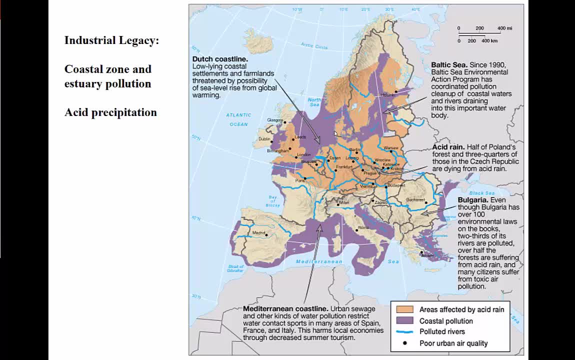 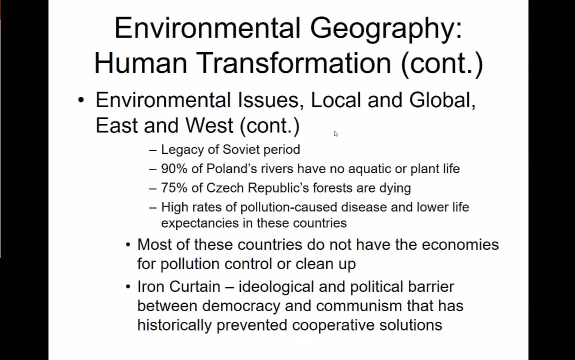 Acid rain in places like Poland and Europe, Eastern Europe, these former Soviet bloc countries, Then air quality issues you know from some of the manufacturing regions in this area, And these just address some of the you know environmental issues that we've dealt with. You know issues from the Iron Curtain, Chernobyl in 86.. 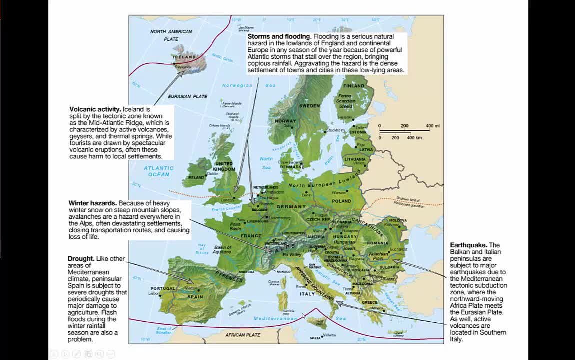 There's also volcanic activity, Because there is a plate boundary that separates the African plate from the Eurasian plate, And then we've got a divergent spreading center up here in Iceland. So you know droughts, earthquakes all throughout the Balkans and in southern Italy. 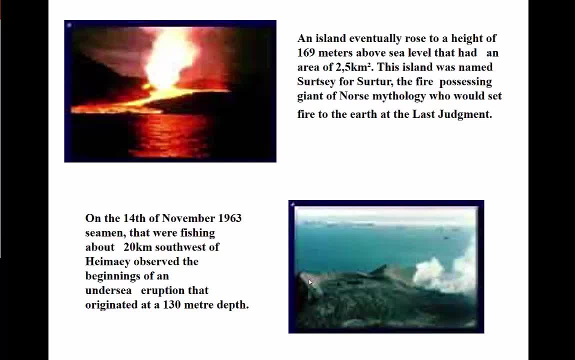 This is a Surtsey in Iceland. So, like I said before, basically Iceland's literally being spread apart through the middle, Because one part of Iceland is on one plate, the other is on another plate. It's at a spreading center or a divergent plate, boundary, and it's being literally spread apart. 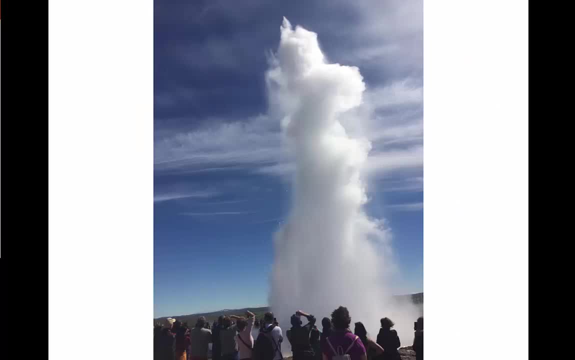 This was pictured in the summer of 2017 when I visited, And they have geysers. There's a national park called Geyser National Park, So you can see a lot of these thermal features where, literally, the land is being spread apart. 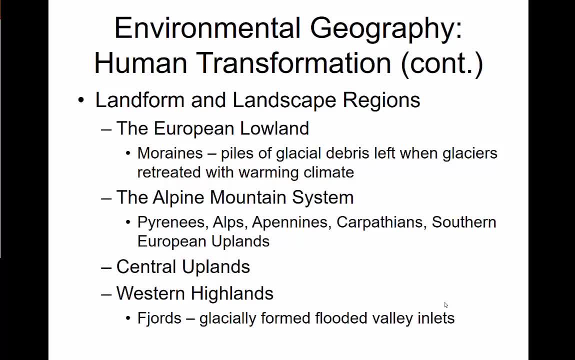 We have moraines which are piles of glacial debris from the glacial retreat. We've got fjords up in northern Europe, glacially formed flooded river inlets, valley inlets. We'll talk about the climate in a little bit. 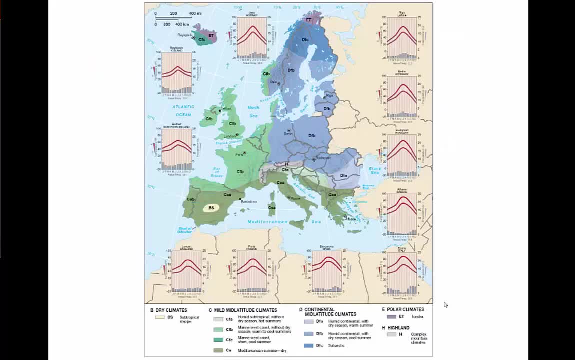 But it's relatively attractive to tourists but can be problematic for agriculture. So you can see the climate regimes we have here. We've got some bees, a little bit of bee in Spain, But you've got your more temperate climate here. 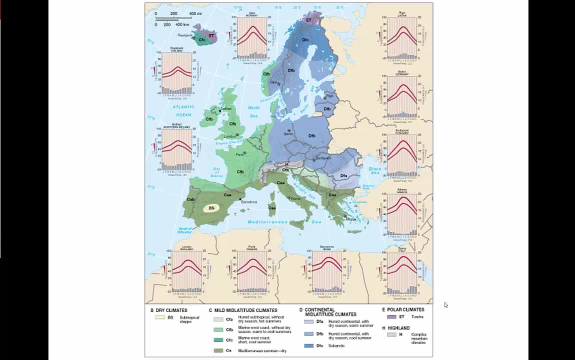 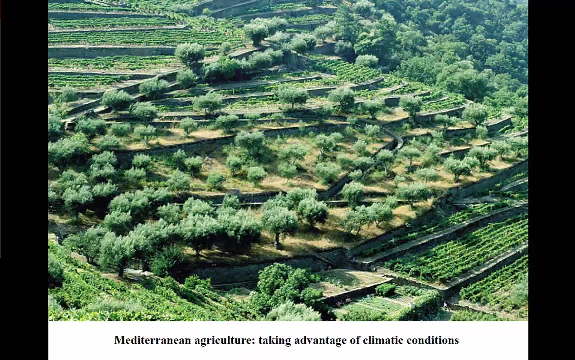 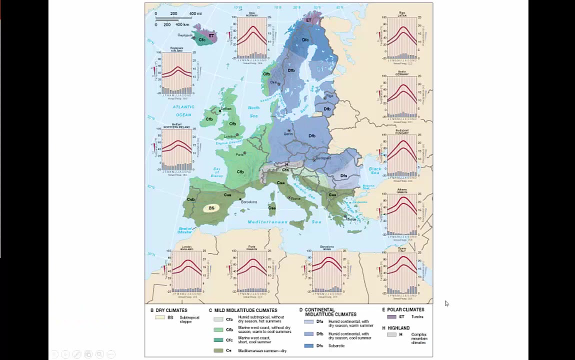 You've got your C's and then you've got some of your D's. So Mediterranean agriculture takes advantage of the climatic conditions. Your palm trees in Dublin, even though when we go back, if we actually look at the latitude of Dublin, 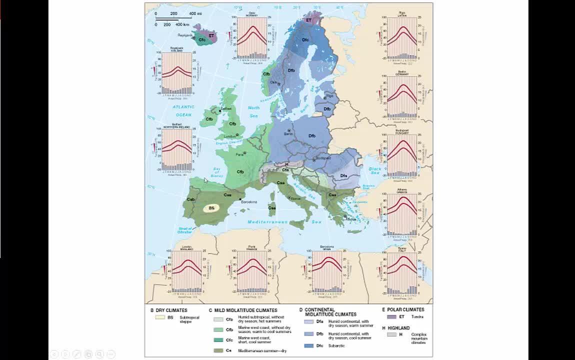 it's relatively high compared to the rest of the United States. New York City is at about 40-41.. So you see Spain here. it's a much different climate regime than we have for the same latitude, But the global circulation patterns that we have are much different. that affect Europe than the United States. 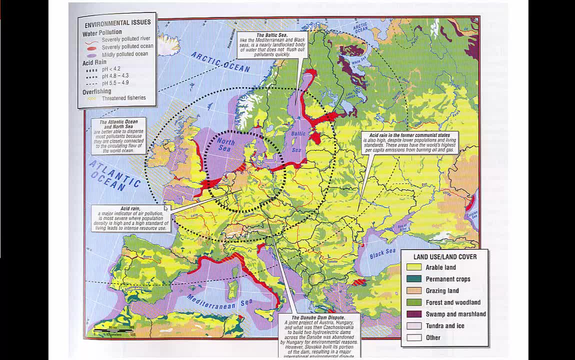 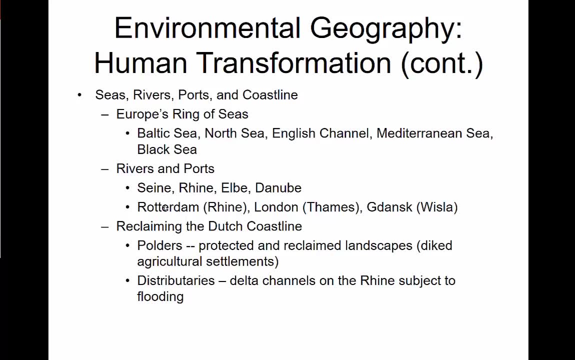 So you can see some of the issues- environmental issues, water pollution- that I kind of expounded on before. Like I mentioned, before rising seas, There's global climate change. That change is going to have a dynamic effect on some of the water bodies. 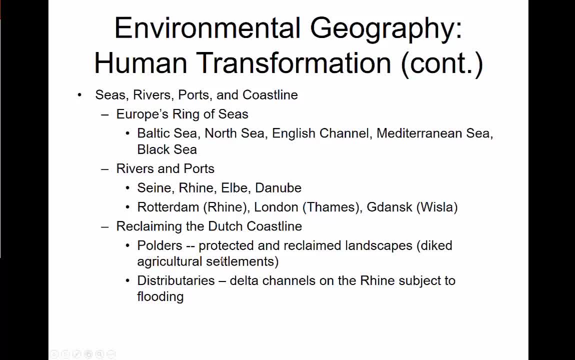 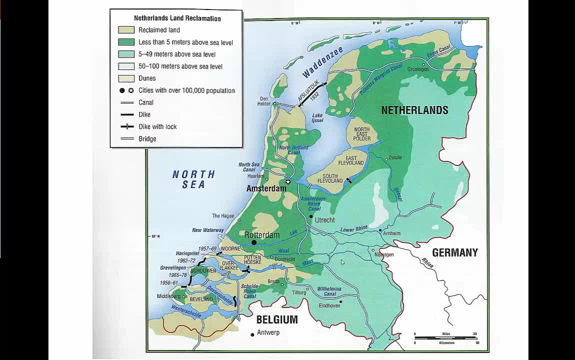 And so we have reclaiming the Dutch coastline and these are called polders. These are protected and reclaimed landscapes And you can see an example of these at a high scale for the country of the Netherlands, Kind of tucked in between Germany, Belgium, into the southwest France. 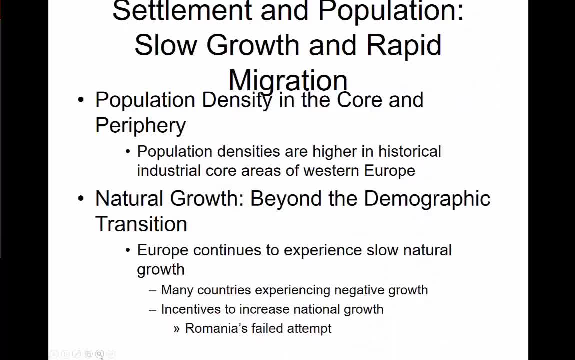 We have population growth. We have population growth in the United States. We have population growth in the United States. We have population density in the core and the periphery. So population densities are higher in historical industrial cores of Western Europe, a little bit lower in Eastern Europe. 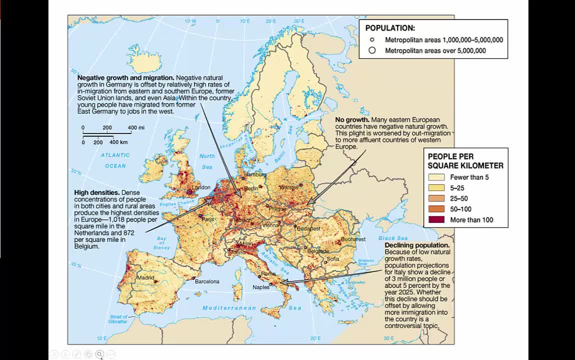 But here's a dot density map that shows where population is concentrated: Very densely populated here in Belgium, Netherlands, Eastern Germany. We have decreasing populations in places like Denmark and Italy. The rate of natural increase is actually going down as opposed to going up. 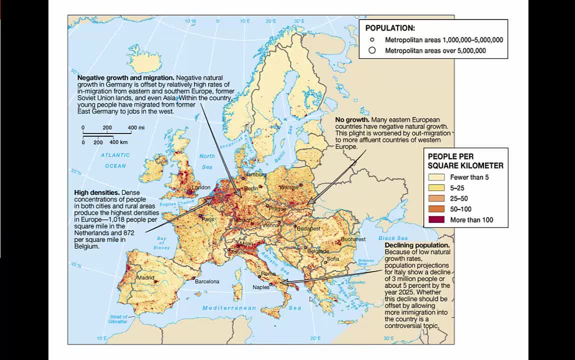 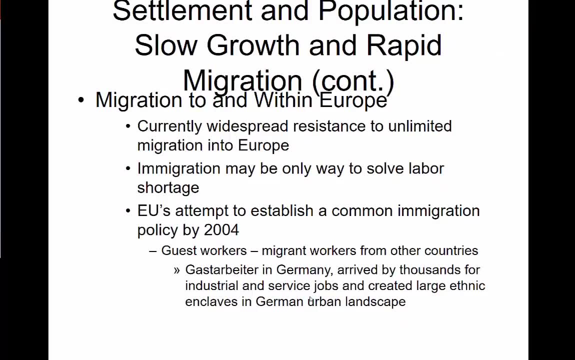 So every day in a couple of those countries more people are dying every day than being born. And then migration: EU's attempts to establish common migration policies- and we see those through to today- Especially this whole idea of distance decay. It's much harder for someone to emigrate to the United States. 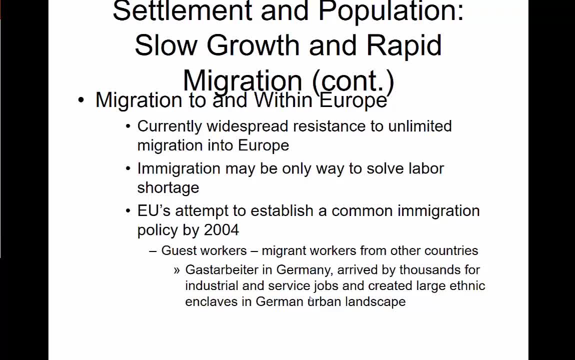 It's much harder for someone to emigrate to the United States. It's much harder for someone to emigrate to the United States. It's a lot easier to do this in Europe because it's relatively close from places like Iraq or Syria or the Middle East. 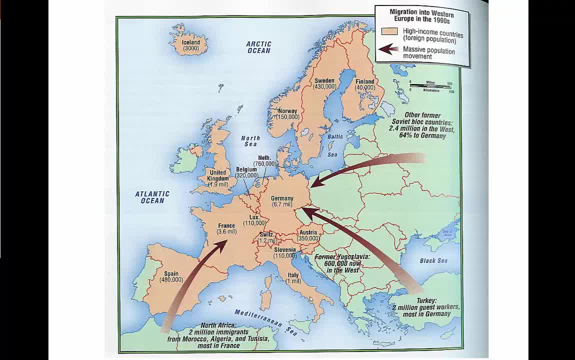 It's a lot easier to do this in Europe because it's relatively close from places like Iraq or Syria or the Middle East, So you can see where some of these people are coming from and going to. and So you can see where some of these people are coming from and going to, and 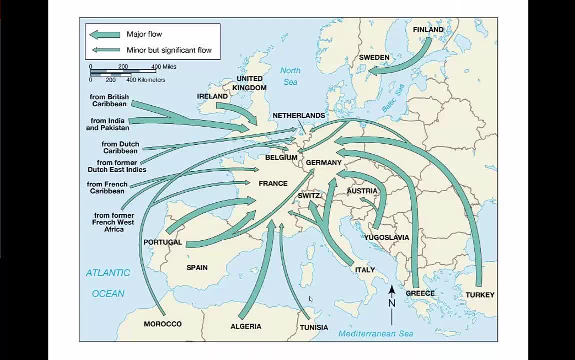 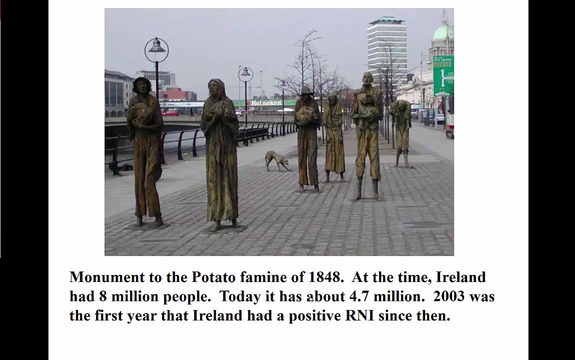 We can still see these patterns persisting today. This talks about it on a much different scale, From the Dutch to the Caribbean, Or to the United States, or to the United States or whatever It's, for a number of reasons. This is the potato famine. This is a combination of environmental as well as government policies. At the time, Ireland had 8 million people. Today it has about 4.7 million. It wasn't even until the 21st century where Ireland had a positive rate of natural increase. 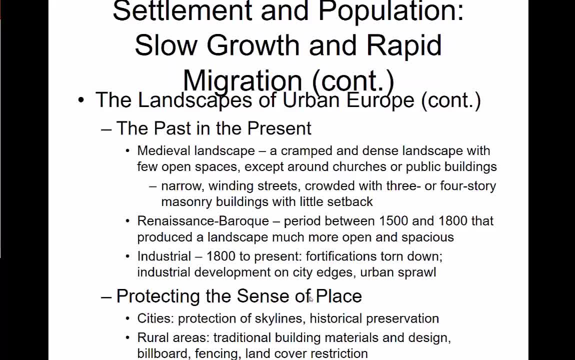 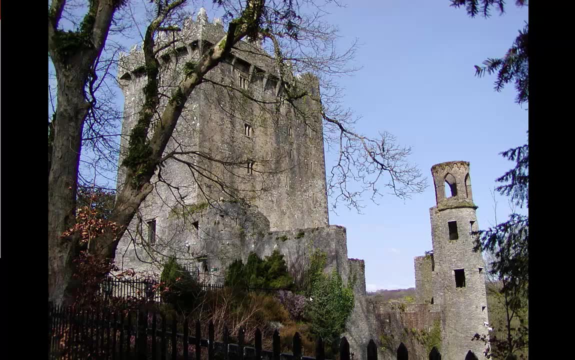 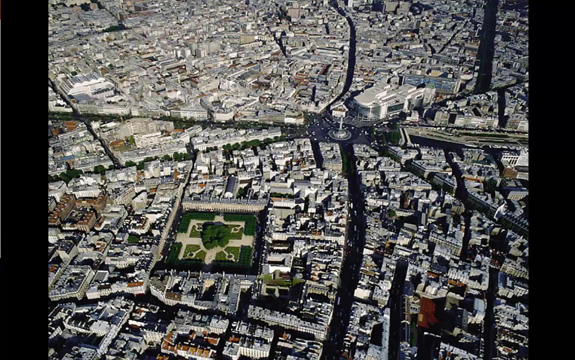 more immigration than emigration. This talks about some of the settlement and growth patterns in the past and how they're looking towards now. This is a picture from Ireland castled and some of the patterns that we've seen there. You can see the high population densities. 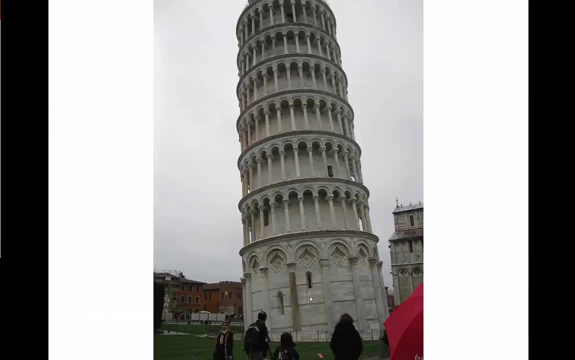 This is a picture of Leaning Tower of Pisa. I was here in March of 2018.. I thought this was really interesting. Pisa was one of the big university centers for all of Europe, one of the oldest universities in Europe. 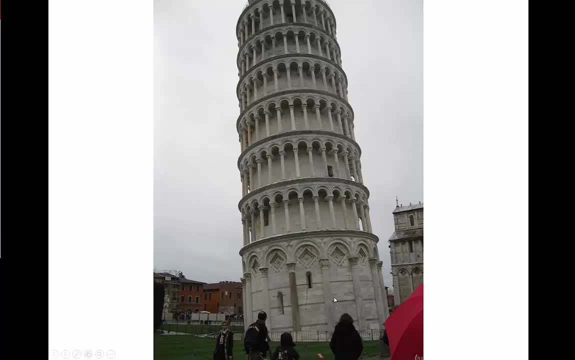 But it's more renowned for this Leaning Tower which was built in the 1300s And then underground subsistence which has kept that going And there's been engineering efforts to kind of take the leaning out of the Leaning Tower of Pisa. 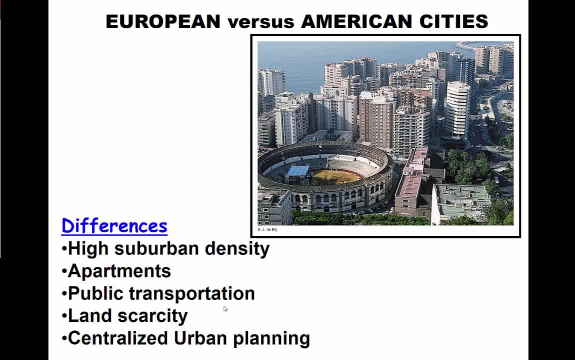 But some of the similarities. it's got a central core suburban ring, Some of the differences between European and American cities, the differences: in the United States we've got high suburban density. In the United States we have a lot less public transportation. 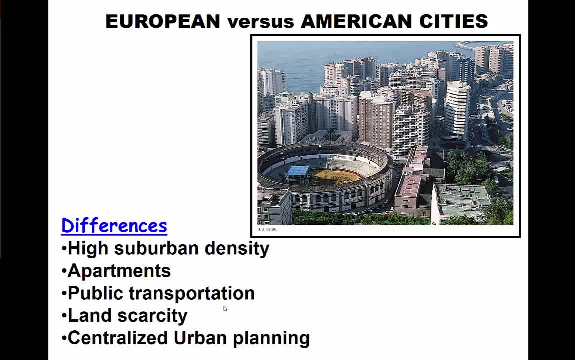 In the United States we have a lot more land, so we're able to just build out instead of taking advantage of or optimizing the land. So we have a lot more land that they do have. So I thought that's much, much different. 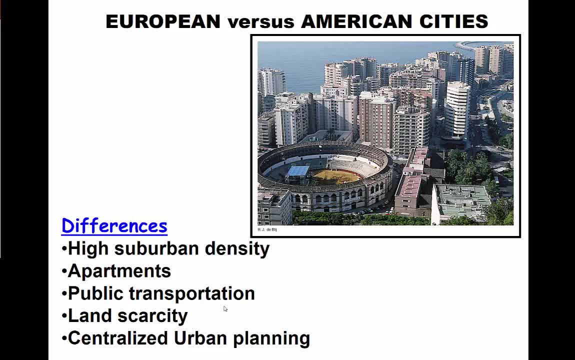 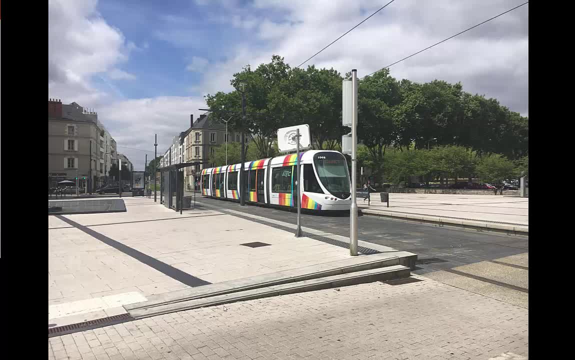 We have these beltways that go around cities. European cities don't have that luxury. I thought this was interesting. In 2017, I went to a city called Angier. It's about 150, 200,000 people and it's got public transportation. 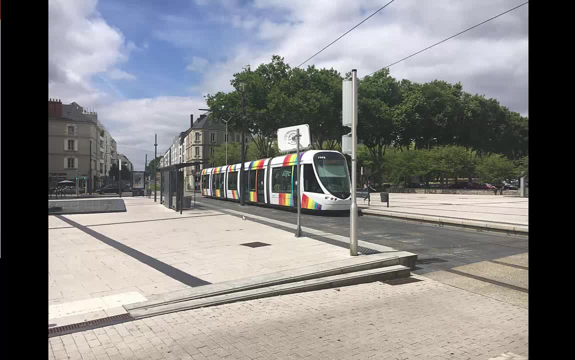 running throughout the city, a public transportation line running throughout the city. So as you can imagine in places like North Carolina or Virginia how much time politics would go into putting in a light rail line or putting in new highways, And it's done relatively easy in these places. 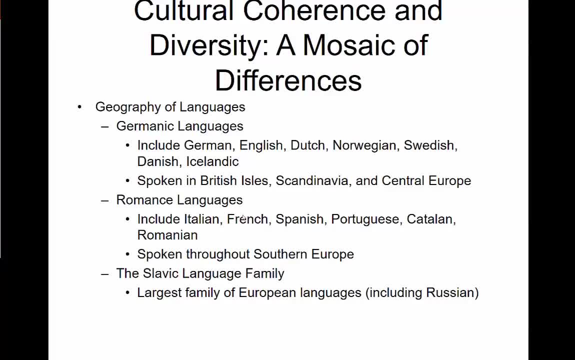 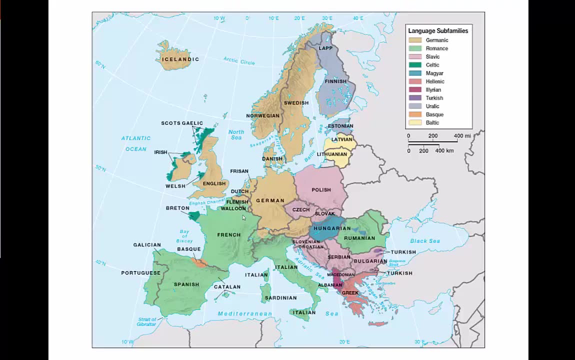 in much smaller places. This talks about the geography of languages And you can see some of these isolated languages here. We have one here called Basque, situated between France and Spain. We can see the different language families throughout. We've got some major, minor. 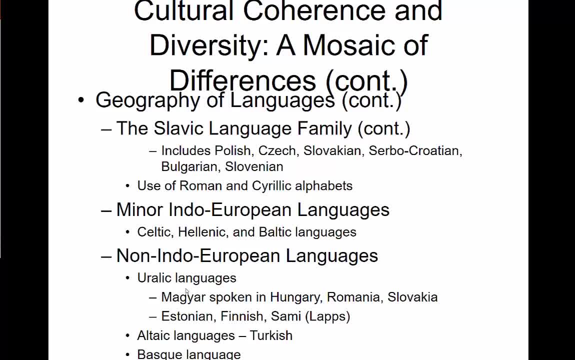 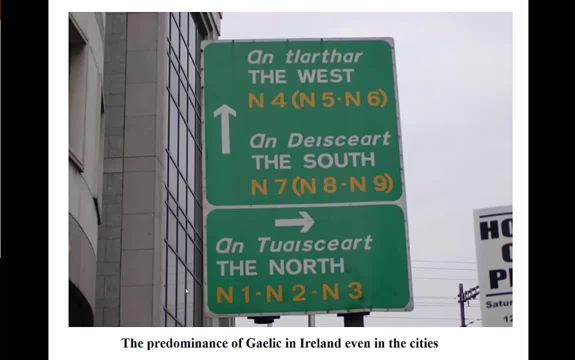 Indo-European from the language family. We've got some major minor Indo-European from the language family. We've got some major minor Indo-European from the other countries. You can see Gaelic or Irish and Ireland And, having been to Europe, a lot of people speak English. 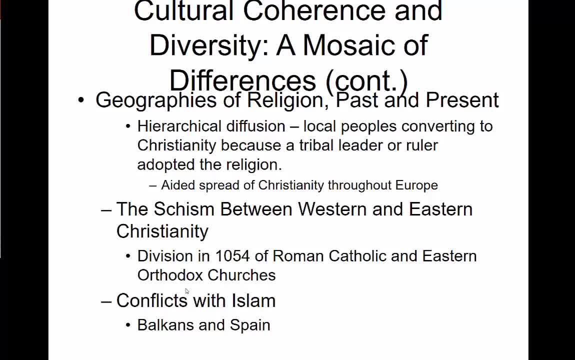 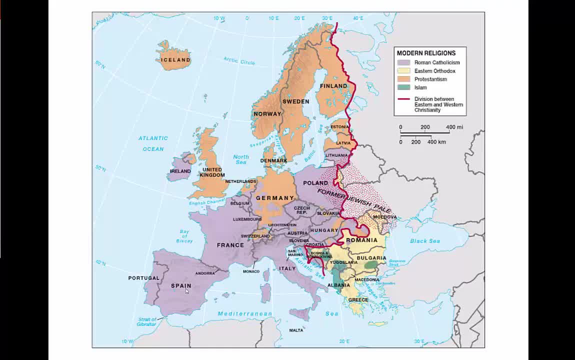 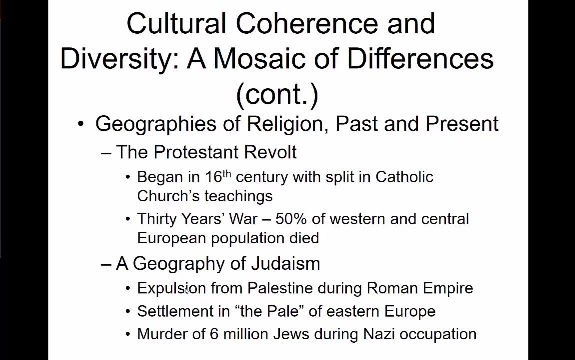 major Indo-European English, which is good for us. English, which is good for us. This talks about the geographies of religions. You can see the different religions. You can see the modern religions: Geography: Judaism, Protestant revolt, Modernism and Protestantism. 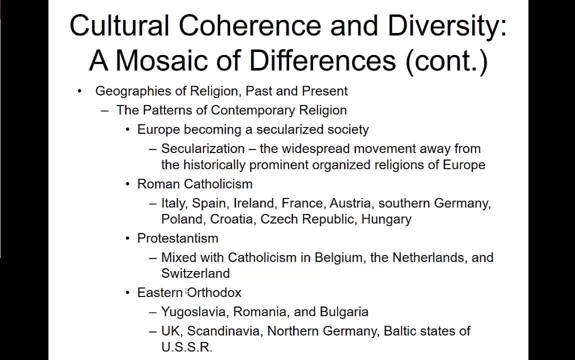 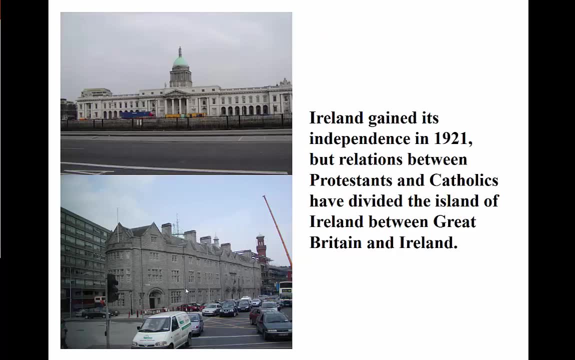 You can see the countries and what they represent in order: secularization of Europe, movement away from historically prominent organized religions of Europe, most notably Roman Catholicism, And we can see some of these interfaith regions these days, like we talked about with Sub-Saharan Africa. 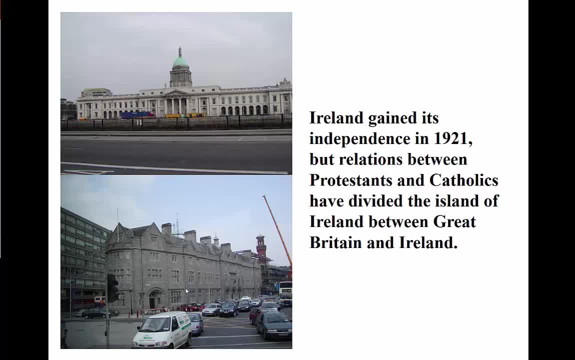 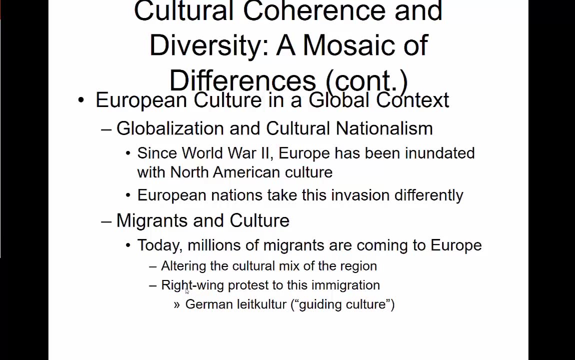 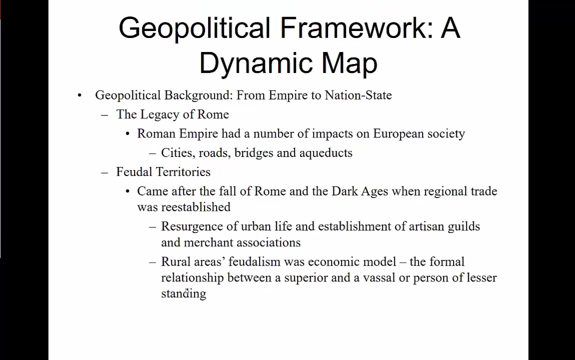 Northern Nigeria, between Islam and non-Islam. We can see with Protestants and Catholics in Ireland, with the separate creation of Northern Ireland which belongs to the Great Britain as opposed to the independent country of Ireland, And we can see the legacy of Rome with the geopolitical background. 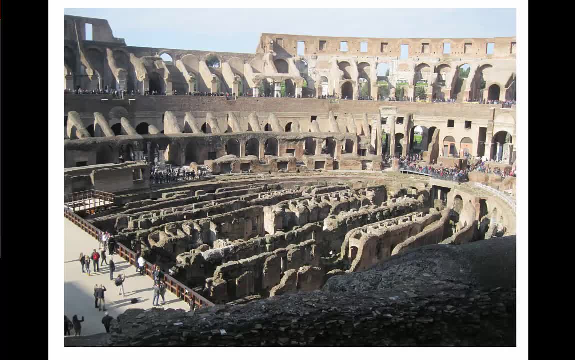 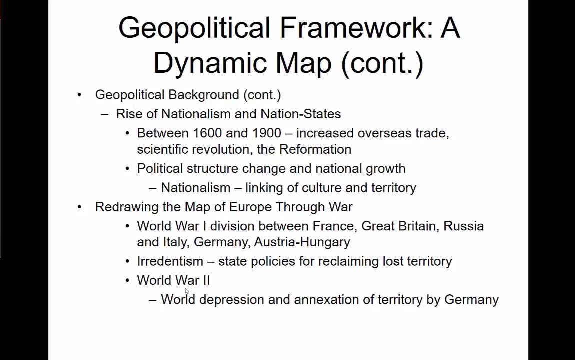 So this is a picture that I took of the Roman Colosseum. This was in March of 2018.. And then the rise of nationalism in nation-states. So between 1860 and 1900, we've got overseas trade. 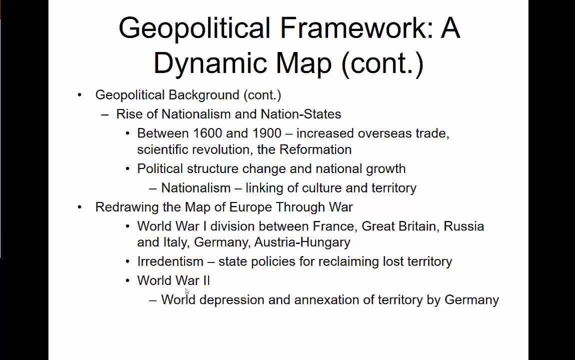 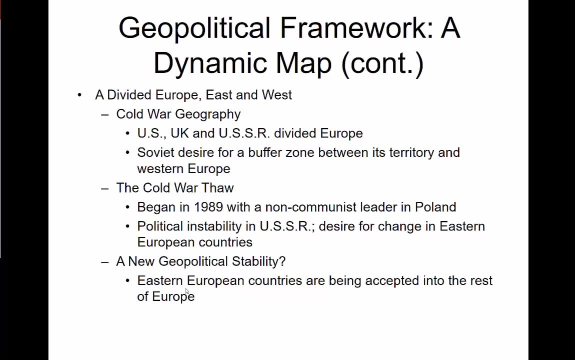 scientific revolution, the Reformation, and then redrawing the map. So, between you know, in the 1900s you'll see countries like Austria-Hungary appear on the map and disappear. Poland will be there and disappear, And we've got the Cold War. 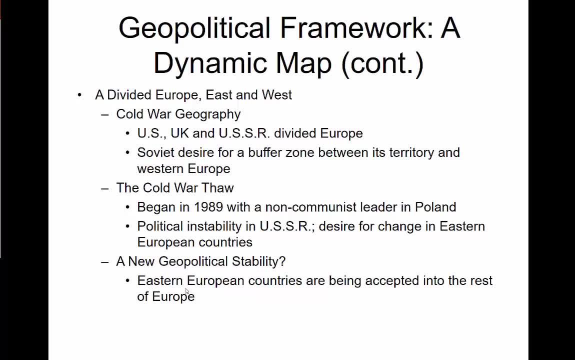 So we've got the US, the UK, the USSR and kind of divided between those who've side with US and UK, and then this USSR, And then this Cold War thaw with the Germany. There used to be an East and West Germany. 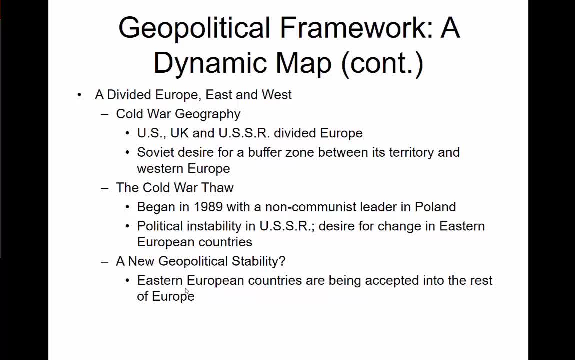 Now there's just one Germany. There used to be a Czechoslovakia, Now it's a Slovakia and Czech Republic. You know, a lot of it's due to this political instability in the USSR. And then how is that going to change things? 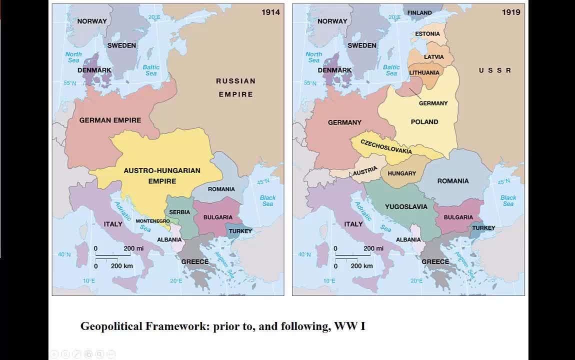 You know, we can see now the breakup of Yugoslavia. So even now we're starting to get these new countries. as a result of those, We've got Slovenia, we've got Bosnia. Kosovo is one of the newest countries in the world. 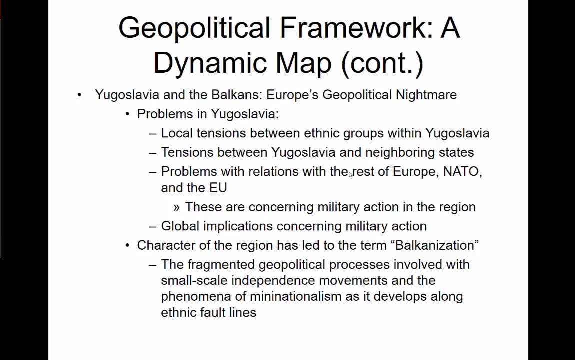 And so some of the problems in Yugoslavia, even to this day. You know the whole like we use the term Balkanization. So this idea of small-scale independence, we'll talk about this a little bit more. with Russia, you know, we have places like Ossetia. 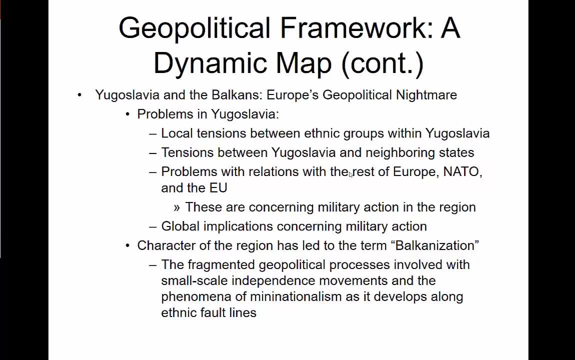 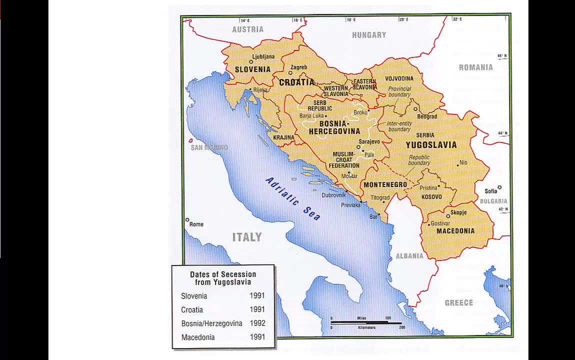 Kazakhstan, which is its own country, but are some of these minor republics going to be declared from parts of those regions in the Caucasus region? So you can see kind of the breakup in, you know, 1991 and where it's moving towards today. 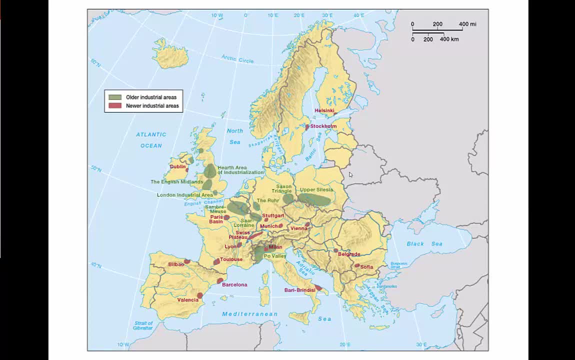 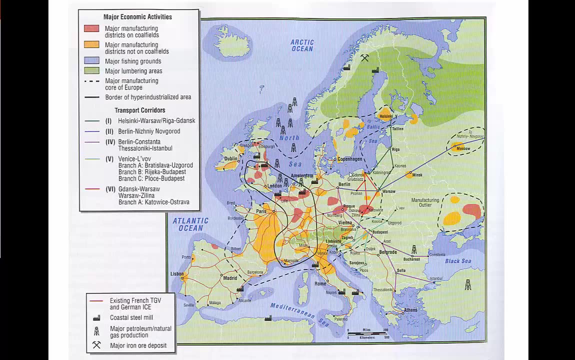 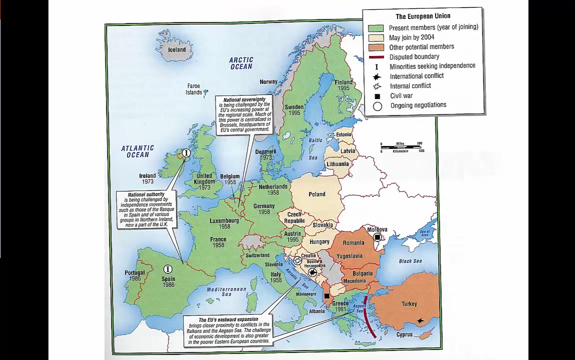 Okay, This talks a little bit about the economic geography, with your newer industrial regions and your older industrial regions in Europe, as does this, And then just getting into the economics, you know, the European Union: is it a good thing? Is it a bad thing?